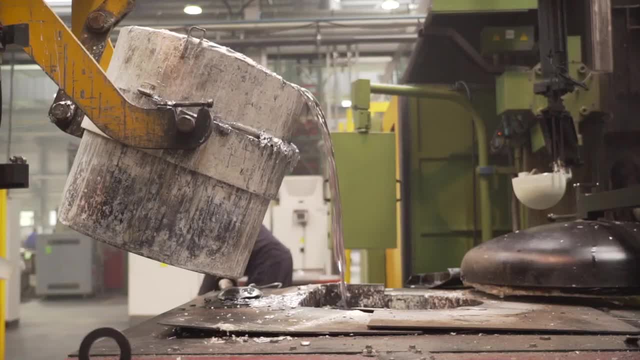 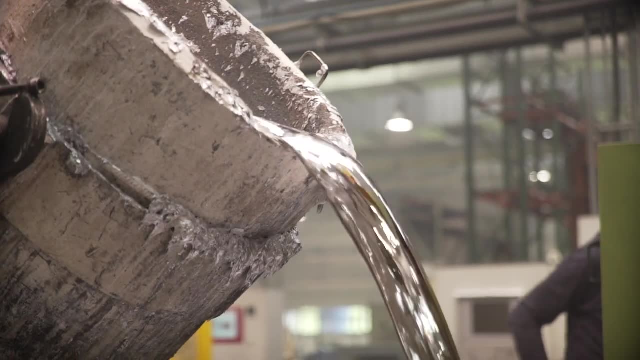 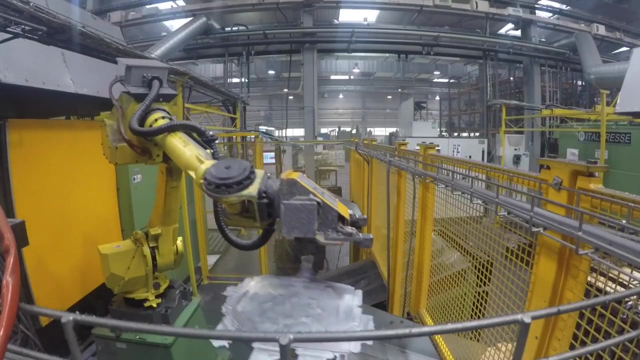 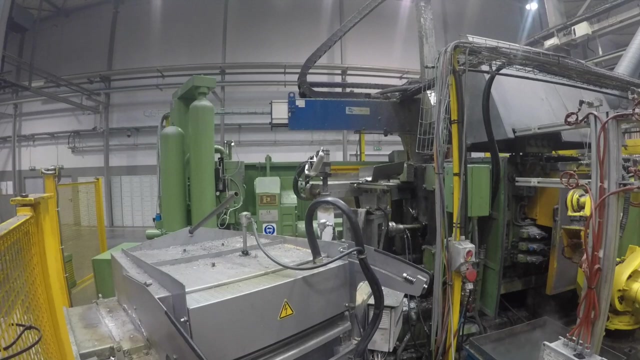 Aluminium is then transferred to the melting stations in order to be inserted to the machine furnaces. Their role is to preserve metal in liquid state. In Metazel foundry, the most state-of-the-art casting technologies are applied. Robot with a precision of 1 gram collects material using a special pipette. 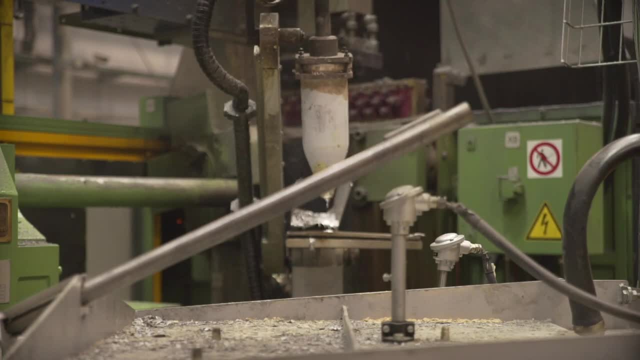 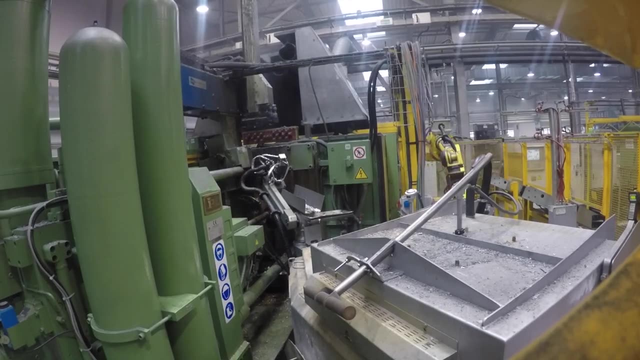 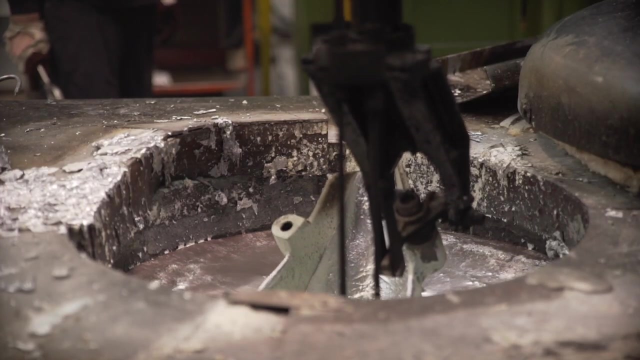 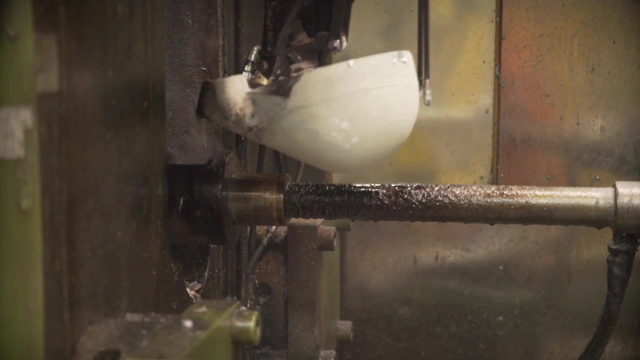 Robot with a precision of 1 gram collects material using a special pipette. The pipette dives beneath the level of liquid aluminium surface. Owing to the above metal injected into the mould is free of contamination resulting from contact with the air. Another method of casting involves pouring onto the filling chamber with a special ladle. 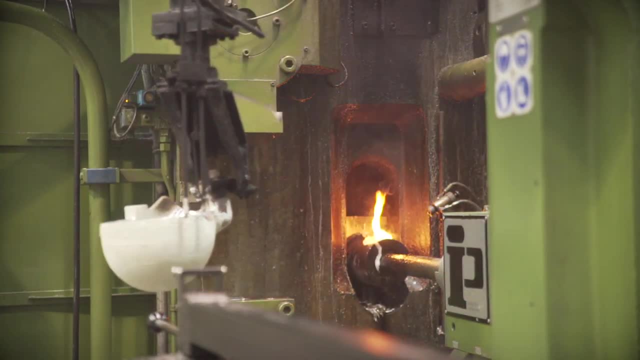 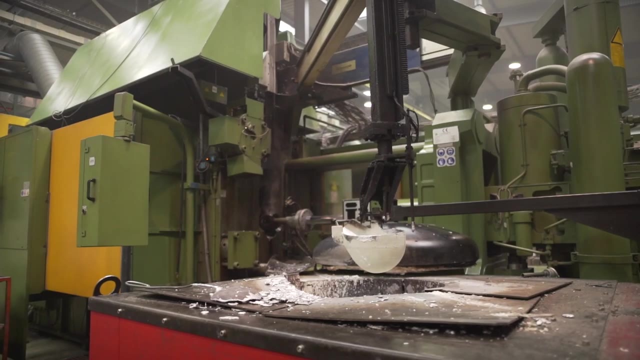 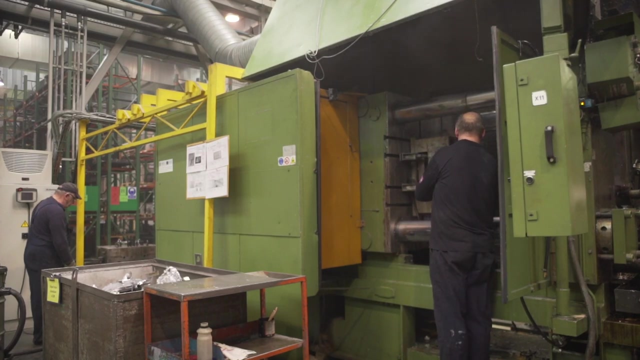 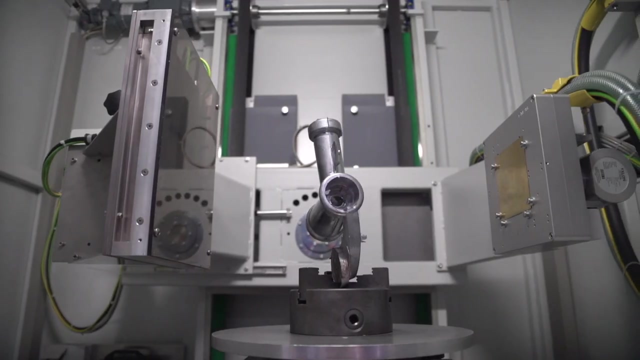 Next, material is forced into the mould and pressed. Next, material is forced into the mould and pressed. Liquid metal fills the entire space inside the mould. Aluminium solidifies and mould opens up. Once we have an aluminium casting, rentgenographic examination is done, which allows to check the metal structure. 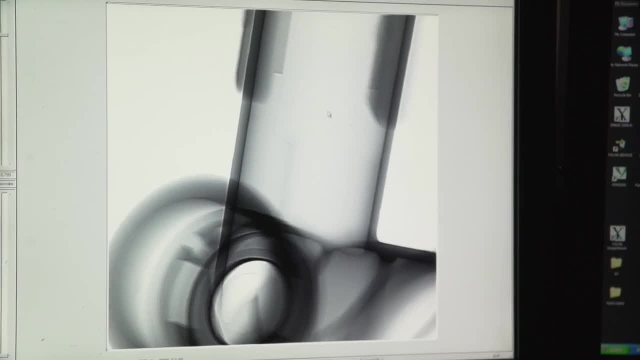 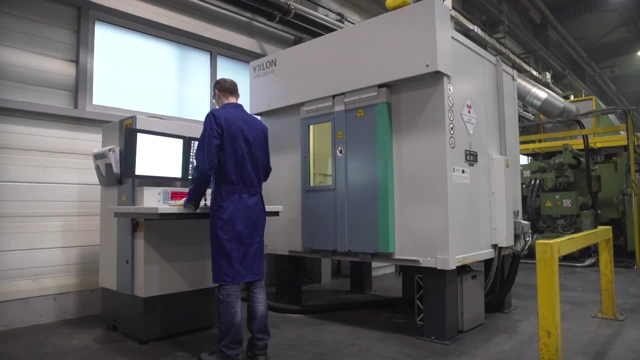 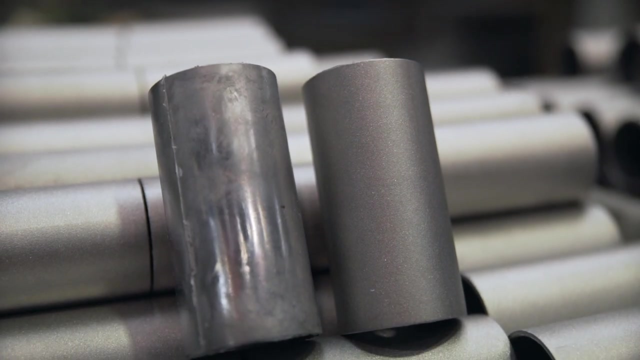 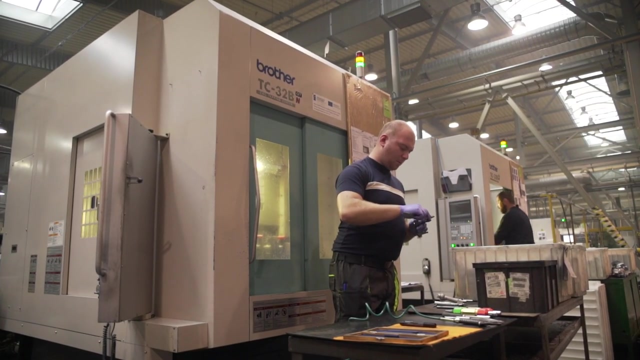 Any contamination, air bubbles or discontinuities in metal structure affect the detail endurance. That is why this examination is so important. Cast detail is purified and subjected to tumble finishing or shot blasting. Next it is moved to the machining department, which is carried out in three axle horizontal and vertical machining centres. 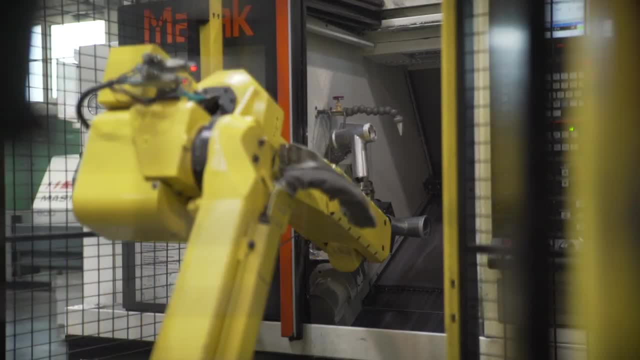 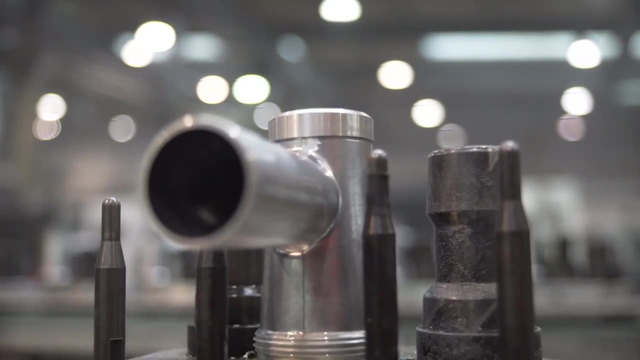 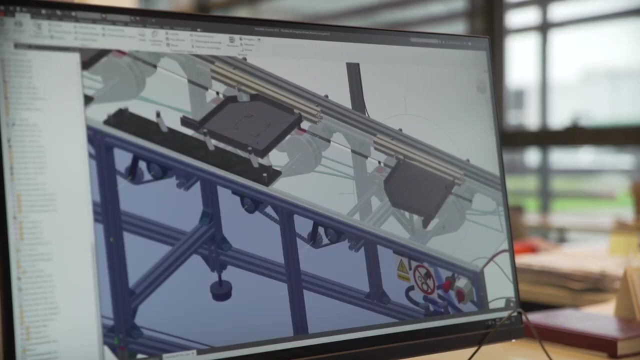 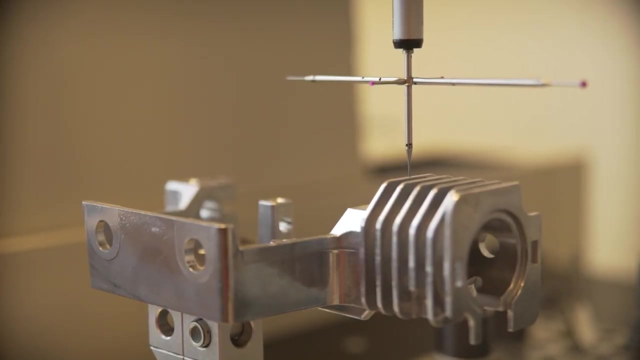 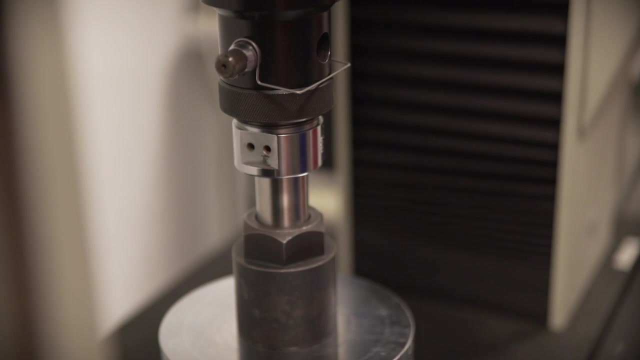 and NC-controlled turning machines, Threads and turning process is performed. Details are milled. Samples of final details are delivered to the control department where the special quality tests are performed: Measurements with the precision of up to 3 microns, endurance and strength tests. 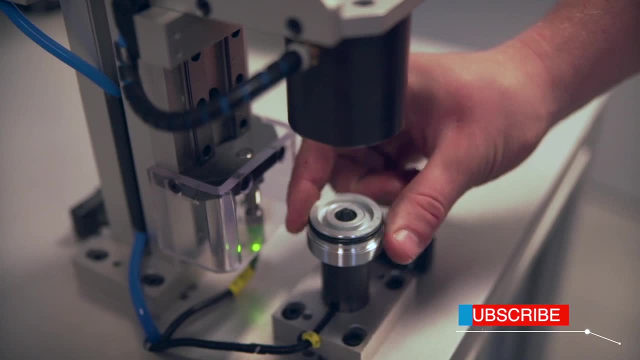 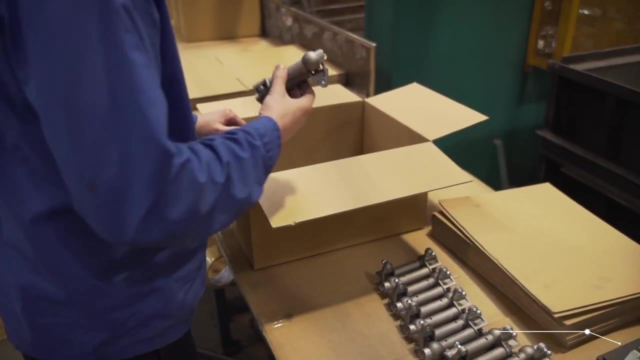 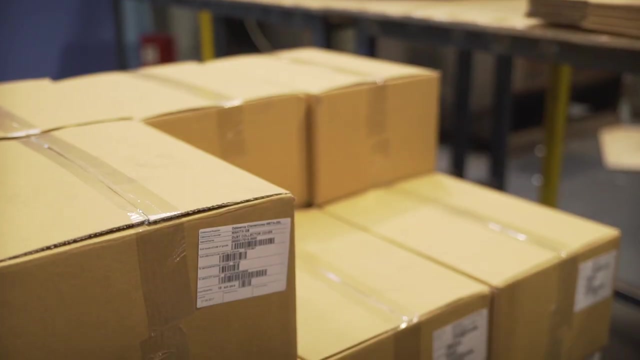 as well as analysis of chemical composition of aluminium is performed. When we are convinced that our die castings meet the most rigorous quality requirements, we send them to the customers.